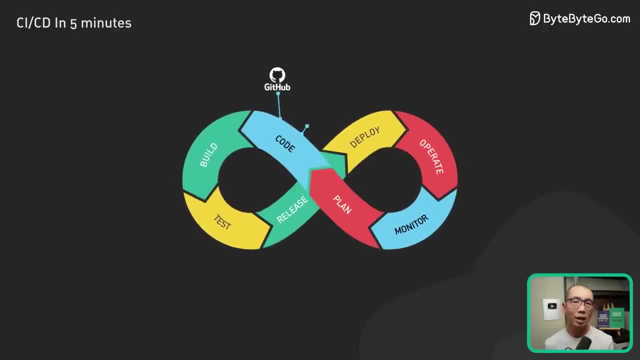 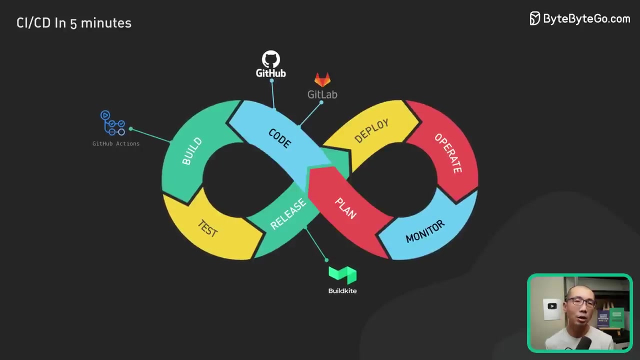 GitHub is a very popular example. It should hold everything needed to build the software. This includes source code, test scripts and scripts to build the software applications. There are many tools to manage the CI process itself. GitHub, Actions and BuildKite are some modern examples. Jenkins, CircleCI and TravisCI are 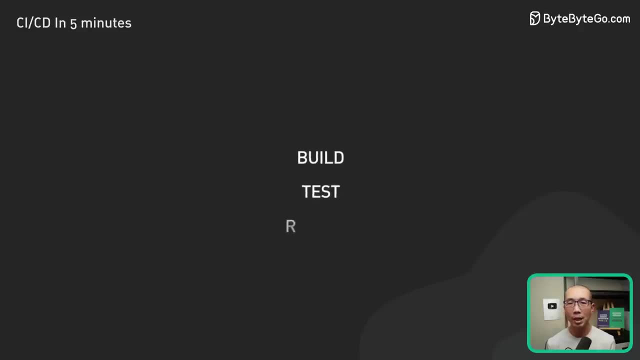 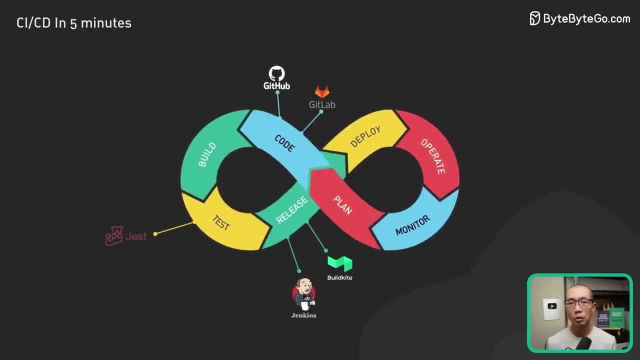 also common. These tools manage the build and test tasks in CI. There are many test tools for writing and running tests. These tools are usually language and ecosystem specific. For example, for JavaScript, JeST is an example of the unit testing framework. 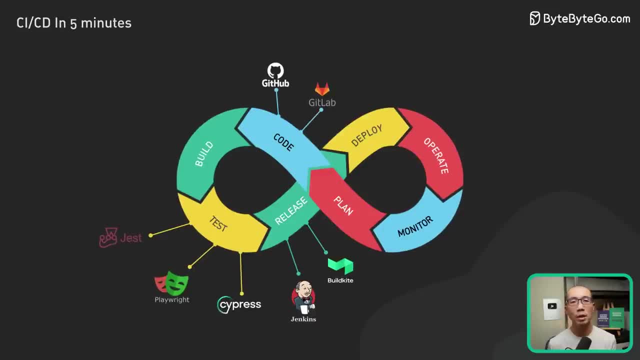 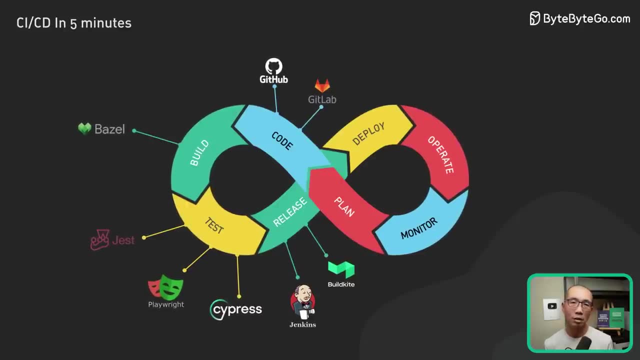 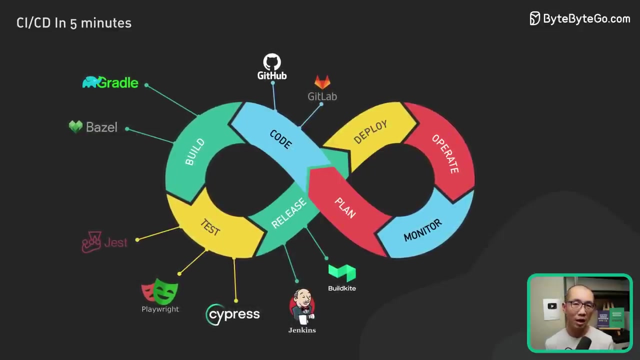 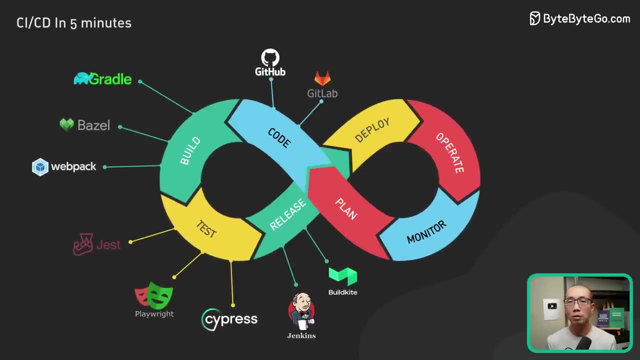 Well, Playwright and Cypress are some common integration testing frameworks for web applications. The build tools are even more diverse and ecosystem-specific. Gradle is a powerful build tool for Java. The JavaScript build ecosystem is fragmented and hard to keep track of. Webpack is the standard, but many new build tools claim to be much faster. 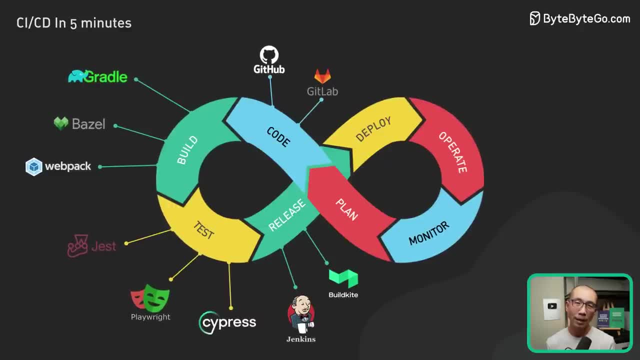 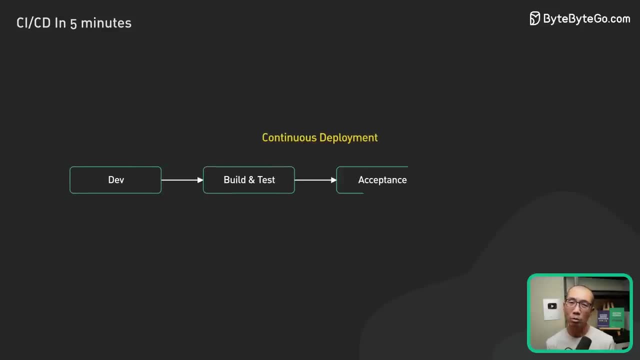 but they are not yet as extensible as Webpack. Now let's examine the CD part of CI-CD. CD is Continuous Deployment. Now, if we're being truthful, real continuous deployment is hard. They do exist, but the practice is not as common as CI. 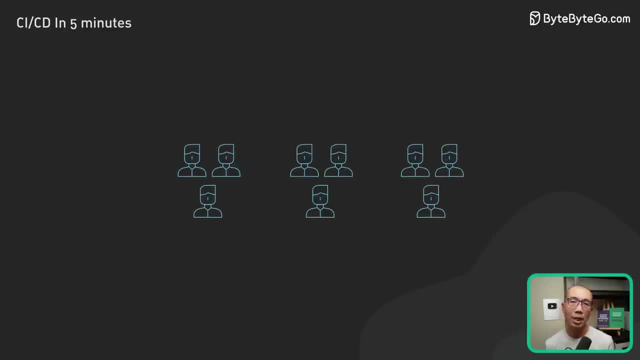 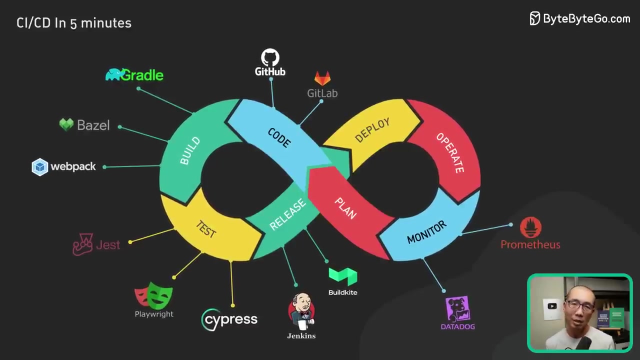 Many teams only practice CD on the most basic types of systems. These systems are usually stateless, like the API or web server tiers. With good production monitoring, these systems could be deployed continuously- continuously with minimal risks. They are stateless and rollbacks are usually quick and harmless. 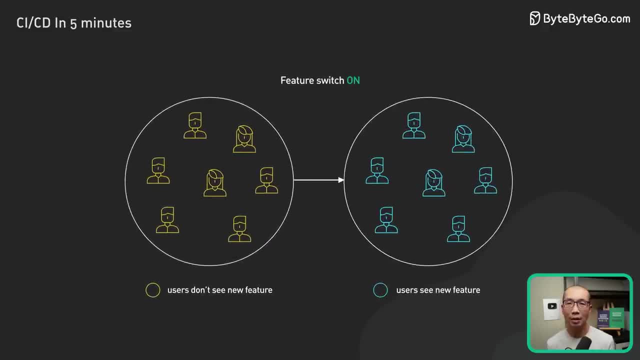 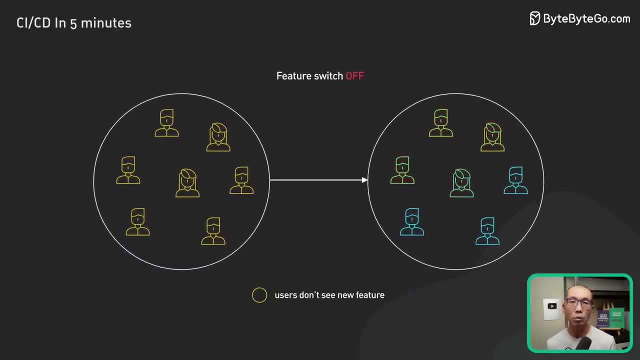 It is also a common practice to wrap new features in feature flags to separate the deployment of the code from the activation of the features. This allows the team to quickly shut up new features if they cause any issues, without requiring a full rollback. Canary deployment is also common practice for products with hundreds of millions of users. 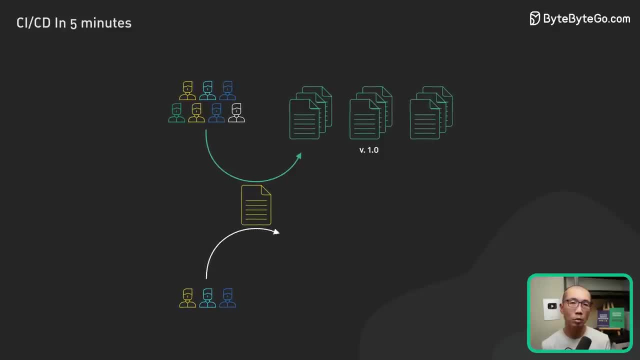 It deploys the new production code to a tiny subset of the power users and staff who both appreciate new features and have the risk appetite to help catch problems before the new code is deployed widely. This allows the team to test the new code in a real-world environment.